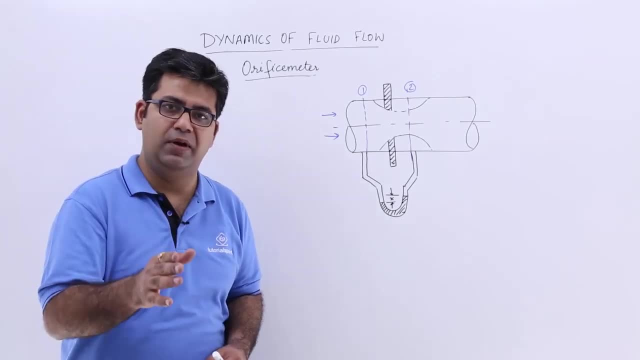 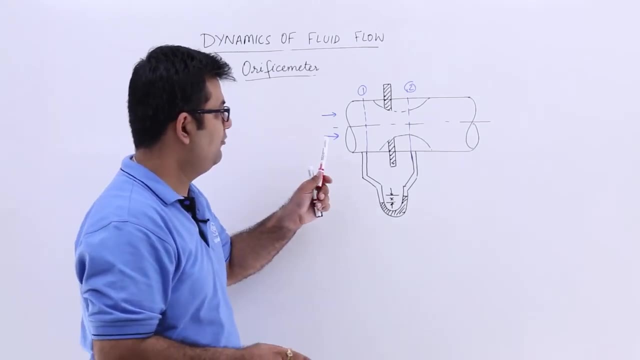 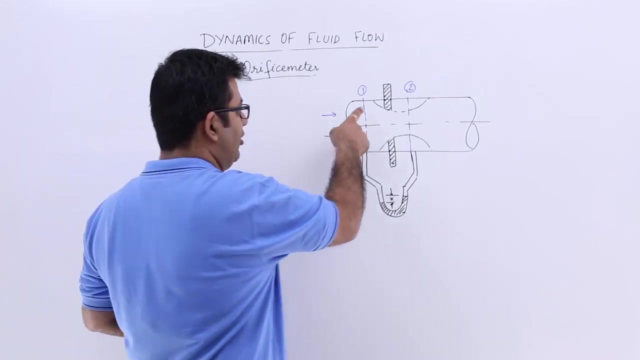 Now, after understanding the concept of Venturi meter, let's have a look at the second application of Bernoulli's equation, that is, the orifice meter. Now, this is how an orifice meter is placed. So, again, it is a apparatus to measure the flow rate through a pipe. You put an orifice meter and this is the orifice plate, The shaded region, this is the orifice plate. 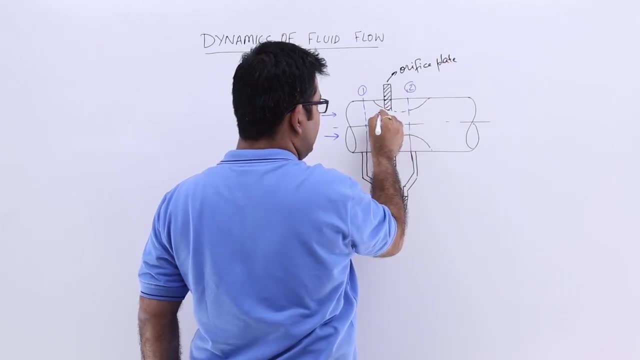 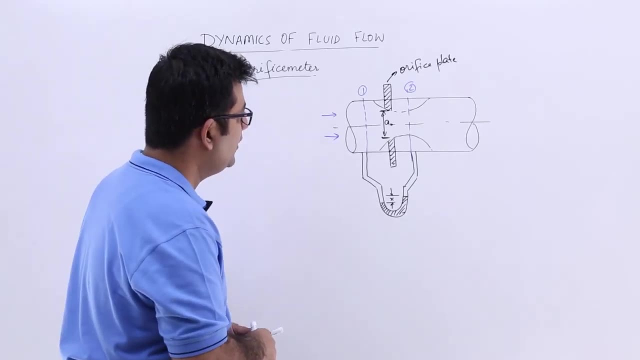 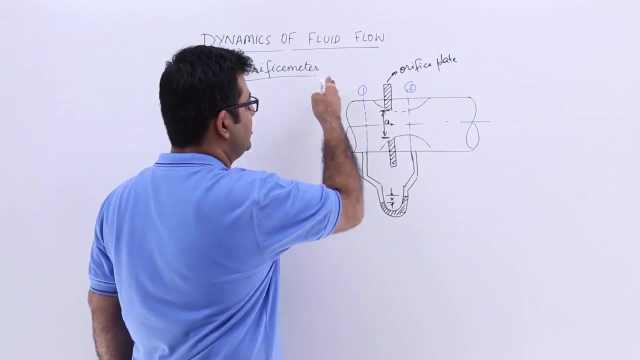 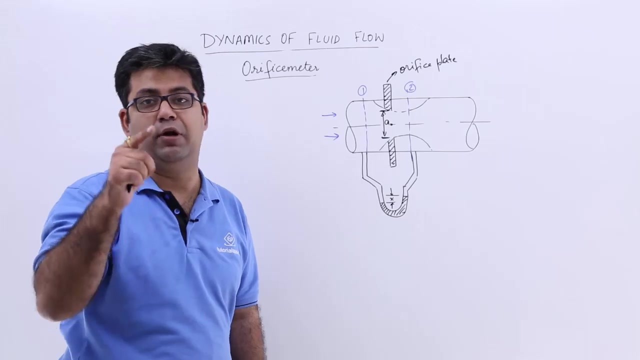 And this is the cross section area of the orifice. Now let's start with it. So we are assuming two sections again. So we are assuming section 1, which is the inlet to the orifice, and then we are assuming section 2.. So section 2 is the section of vena contracta. So I will 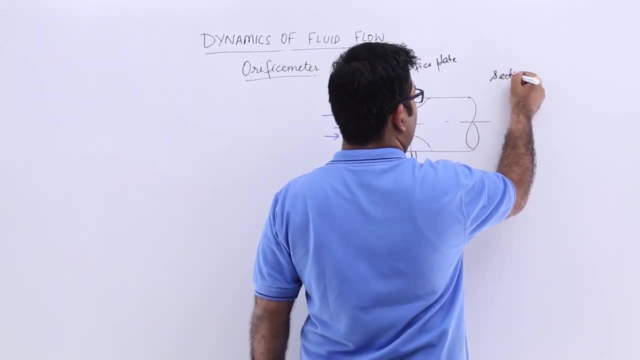 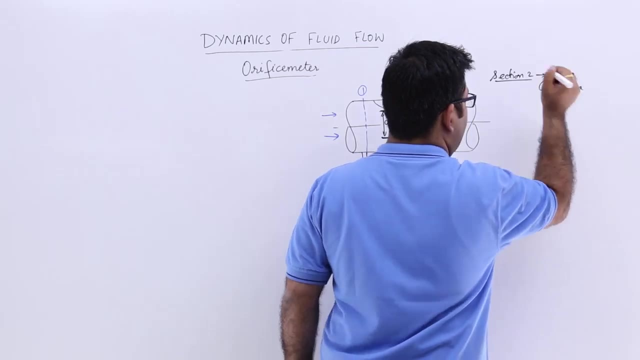 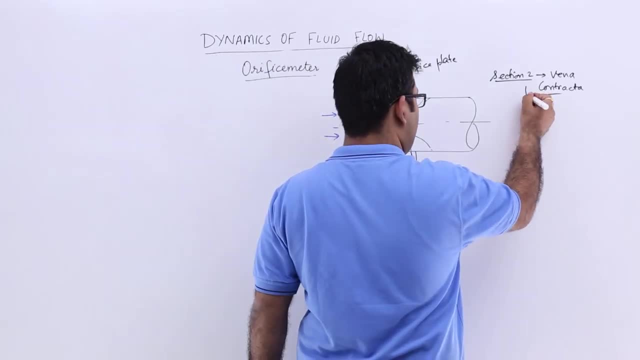 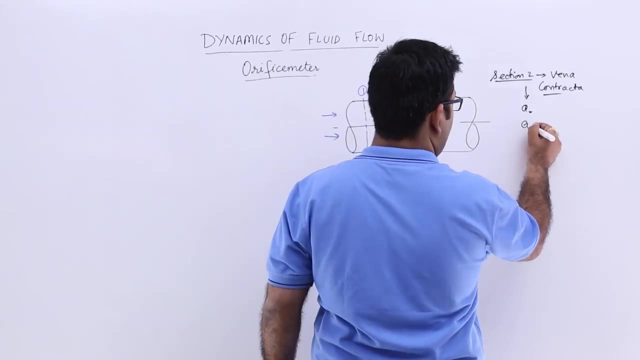 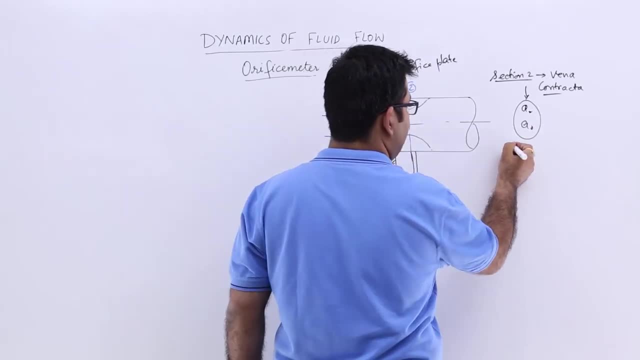 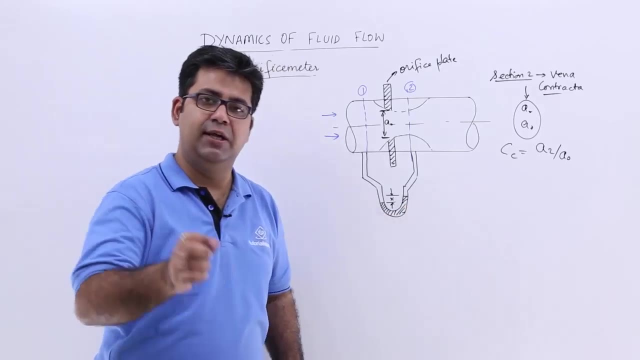 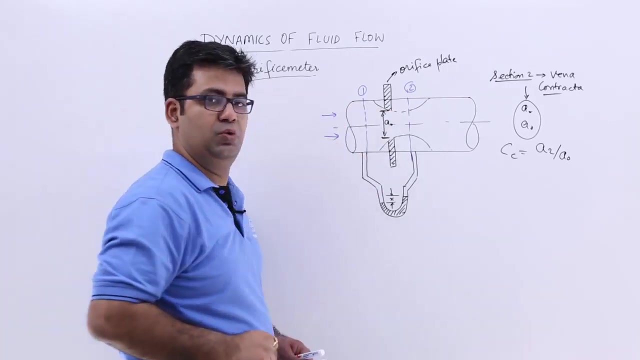 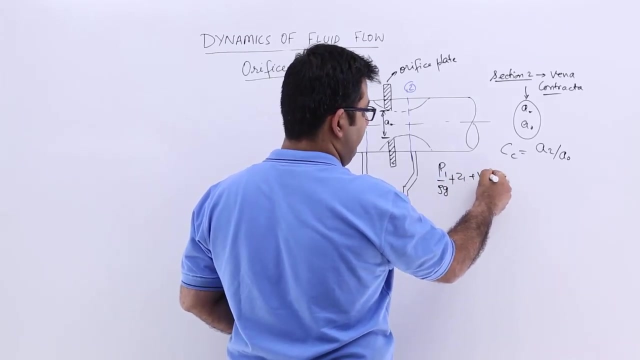 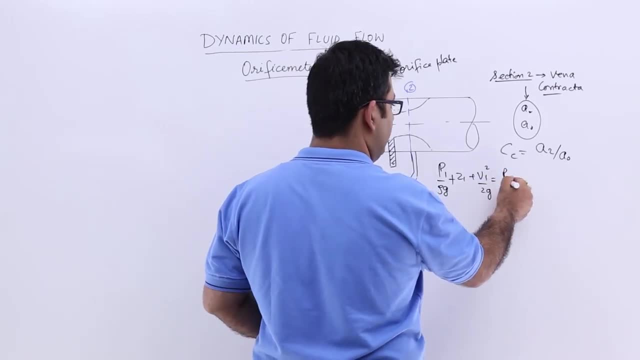 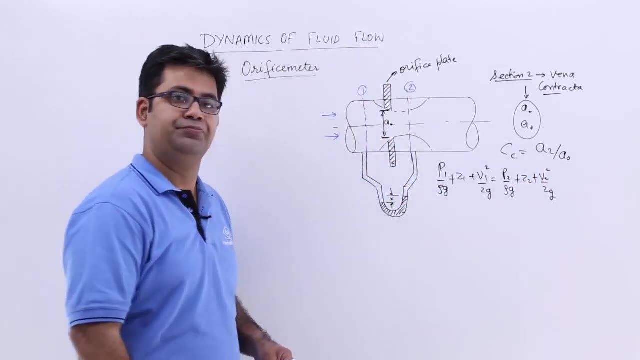 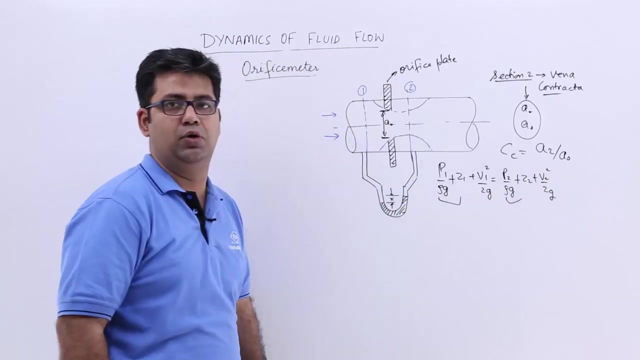 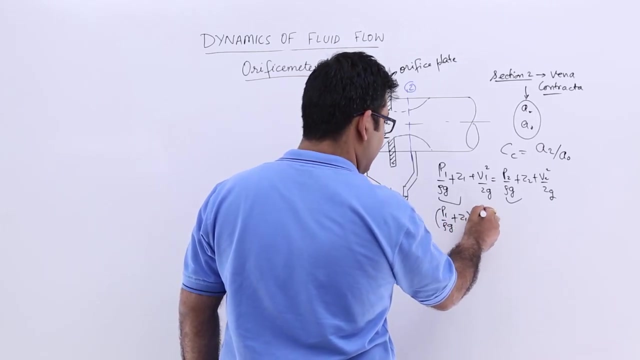 upon 2g is equal to p2 upon rho g plus z2 plus v2 square upon 2g. ah, lets combine this and this and take it on one side and take all the velocity heads onto the other side, so you will get p1 by rho g plus z1 minus p2 by rho g plus z2 is. 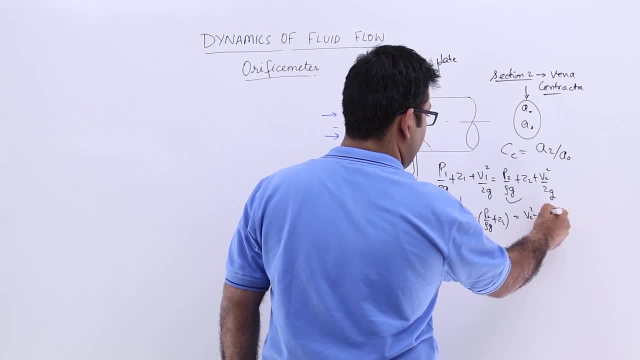 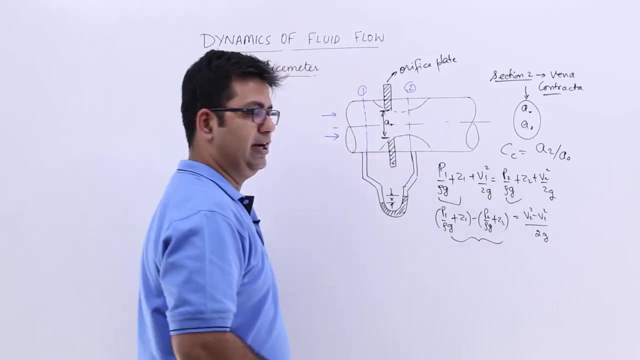 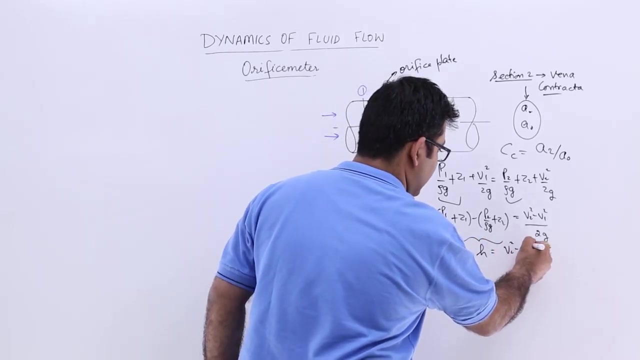 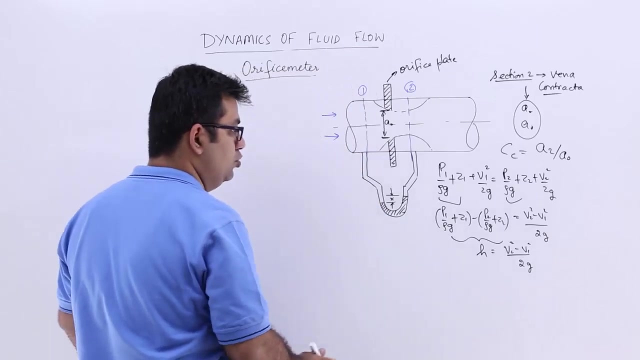 equal to V2 square minus V1 square upon 2G. So again, this is the pressure head, or you can say the piezometric head difference. So this would be: H is equal to V2 square minus V1 square upon 2G. From here I can calculate the value for V2.. So V2 if I just put down the square. 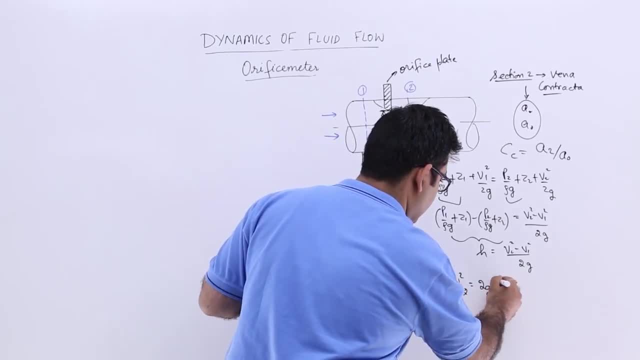 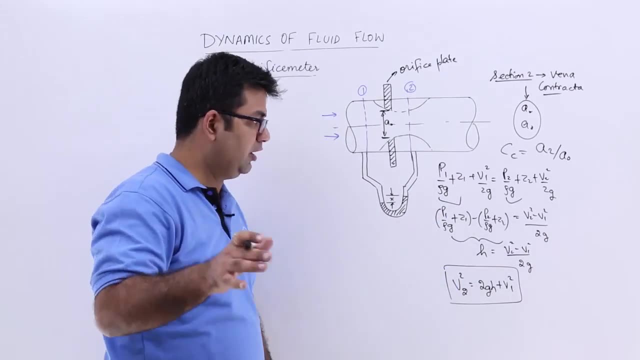 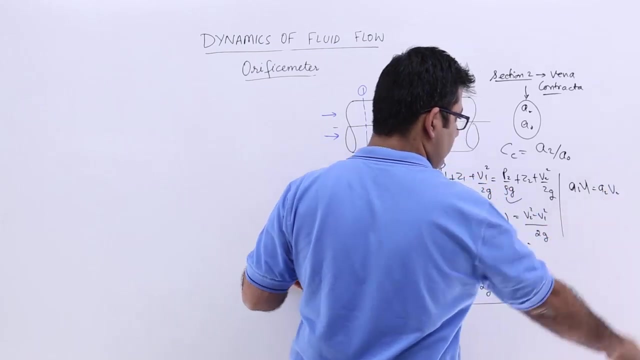 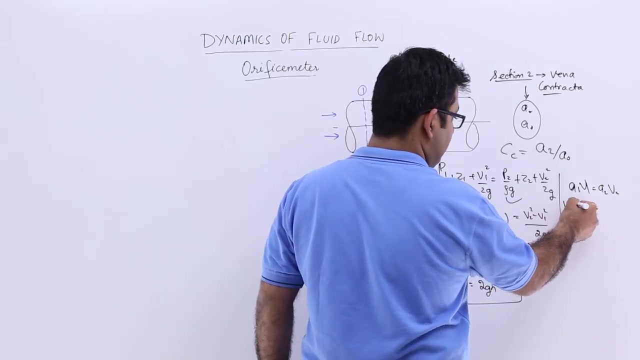 value, I will get 2GH plus V1 square. Now let us apply the continuity equation. Continuity equation says A1- V1 is equal to A2- V2.. So from here I can say that the value for A1 or V1 in terms of the variables would be A2- V2 upon A1.. 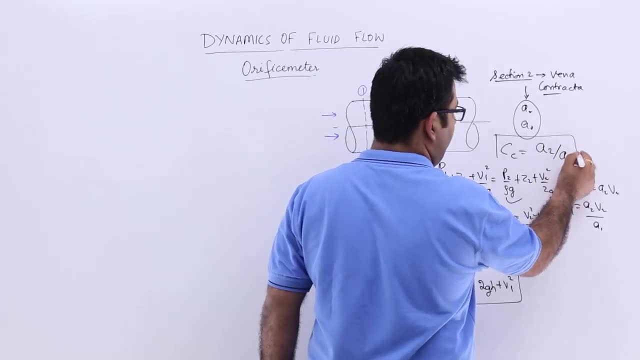 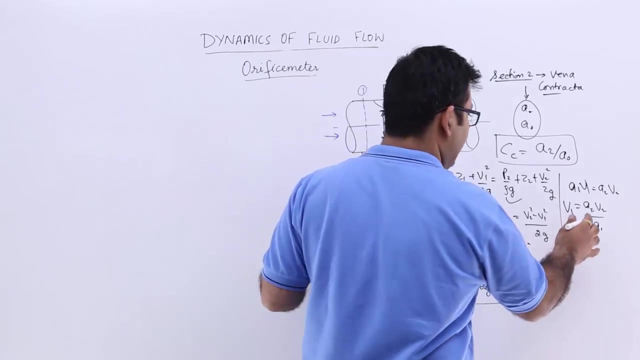 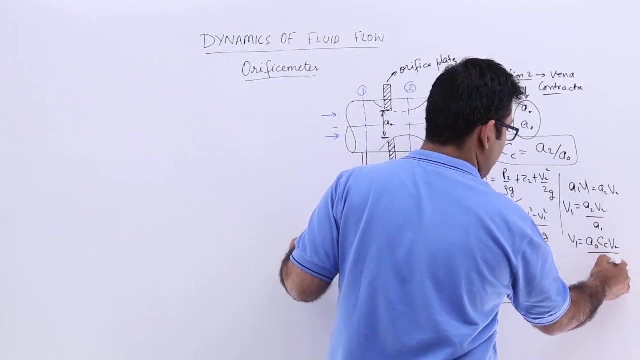 Now, what is the value of A2?? The value of A2 can be found out from here in terms of the coefficient of contraction and the cross section area of the orifice. So you will get V1 is equal to A0 into Cc, into V2 upon A1. So let us substitute that value into this. 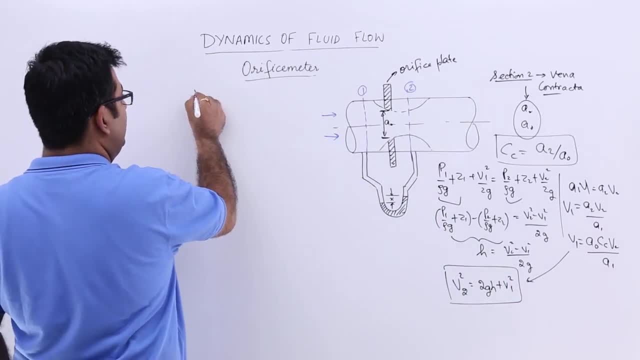 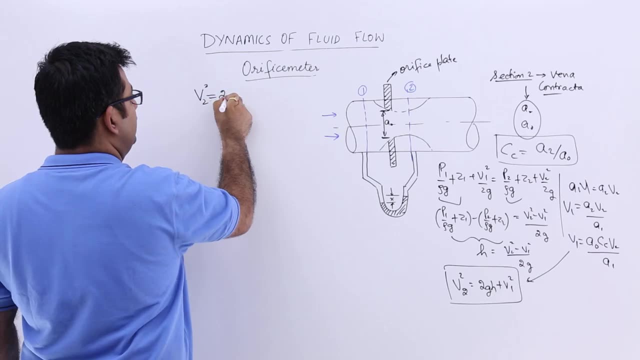 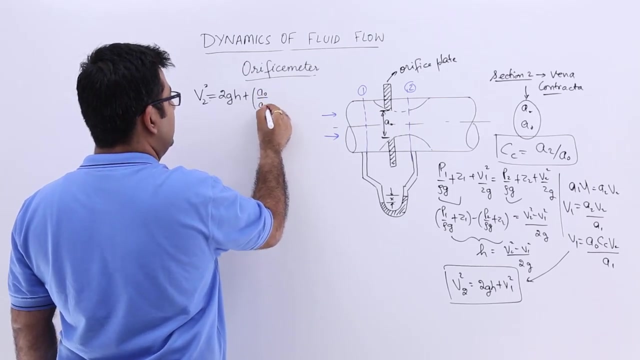 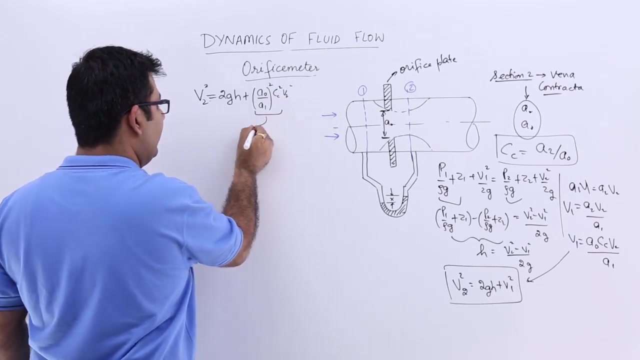 equation. So when you do that you get a value which is V2 square minus V1 square minus V2.. So this would be equal to 2GH plus. I have put down all those values over here. so you will get a0 upon A1 whole square, Cc square into V2 square. So I will bring this entire 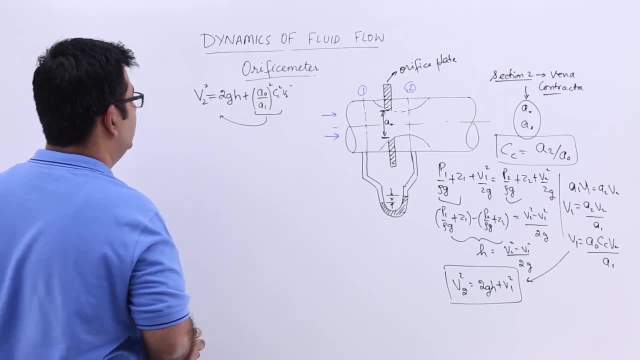 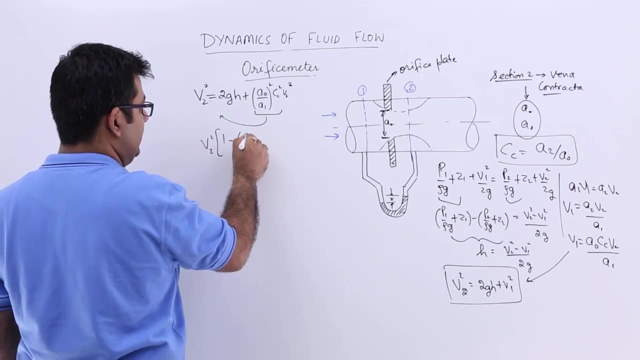 value on the left hand side. okay, So I will get V2 square as common 1 minus a0 into B2.. Let us substitute that. Let us substitute that. We will get Cb into 1 minus Cb. Let. 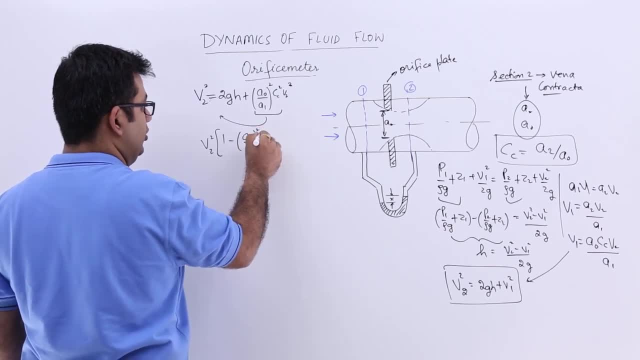 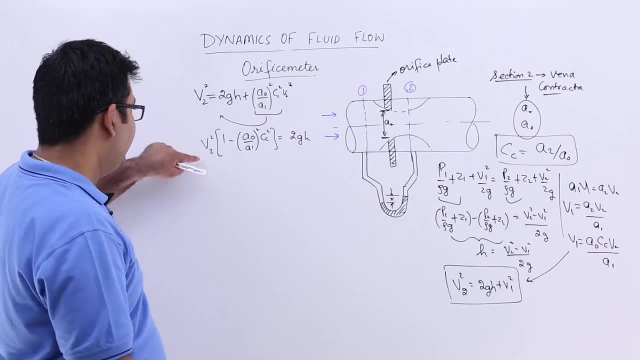 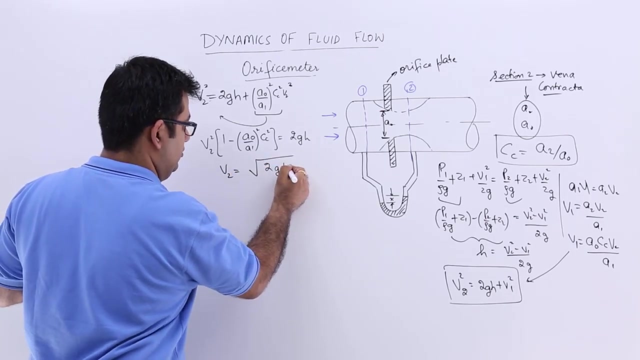 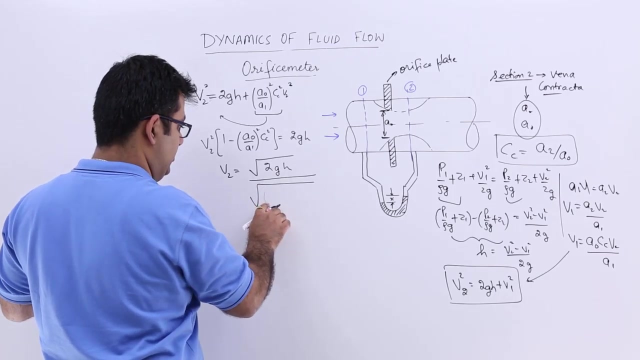 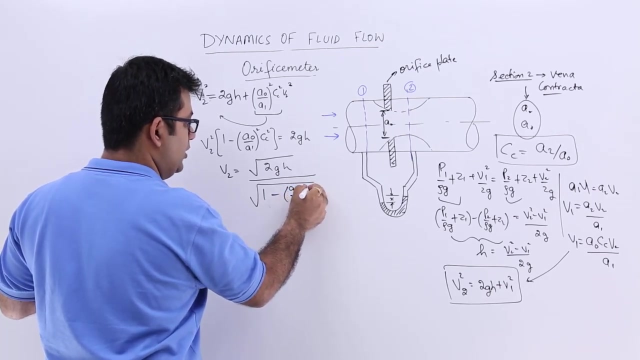 a0 upon a1 whole square into cc square is equal to 2gh. okay, from here I can get the value for v2 very easily. so v2 would be equal to under root. 2gh upon this would be under root. let's get rid of the bracket 1 minus this will be a0 upon a1 whole square into. 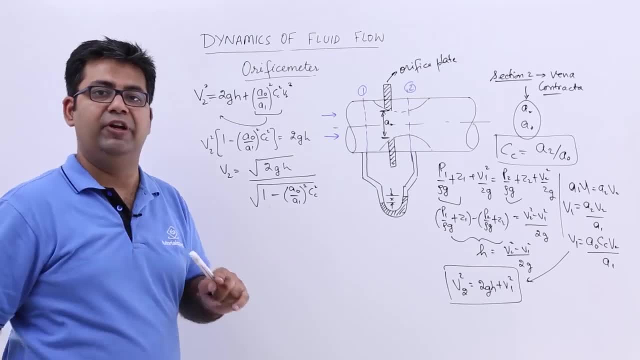 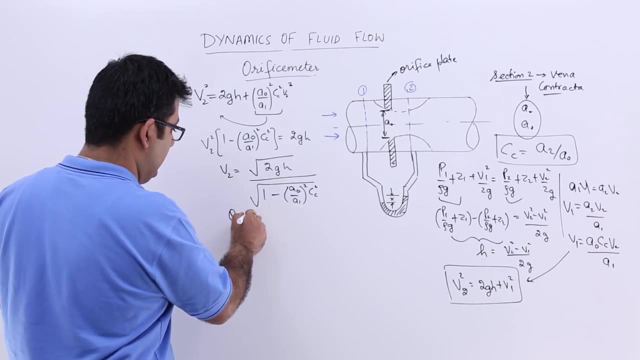 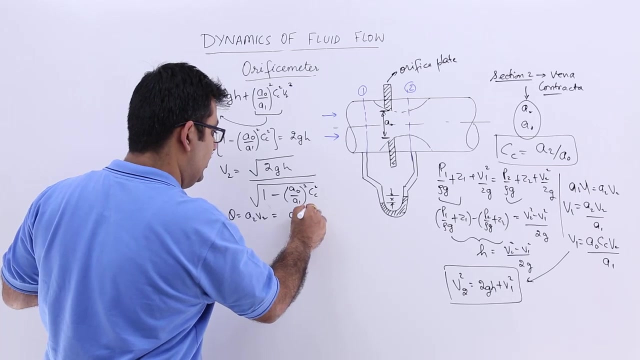 cc square, so this is the value of v2. so if I apply this and find out the value for Q, so Q was a2 into v2, so I'll put v2, so you'll get a2, into under root, 2gh into cc square, so I get a1, whole square, into cc square. let's get rid of. 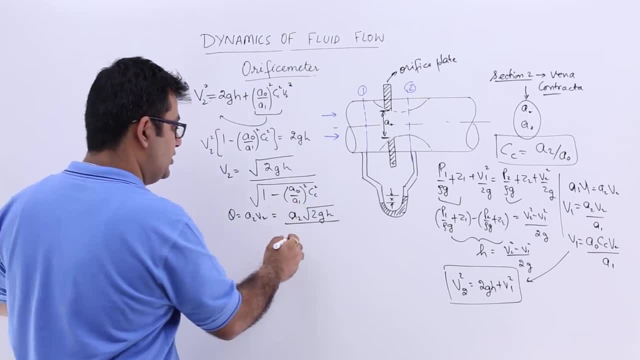 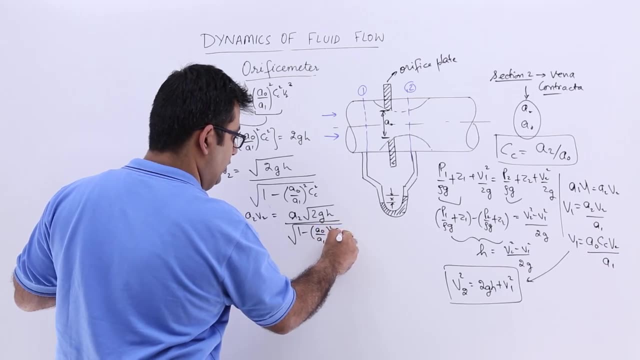 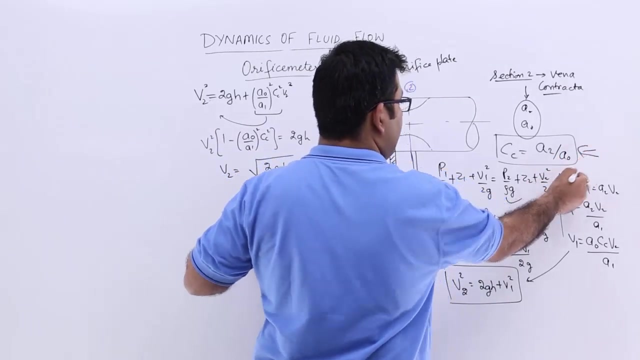 the bracket 1 minus this will be a0 upon a1 whole square into cc square. so this is the 2gh upon all this, that is, 1-a0 upon a1 whole square into cc square. right now I can put the value for a2 from this equation, that is, a0 into cc, so I will replace that. so you will. 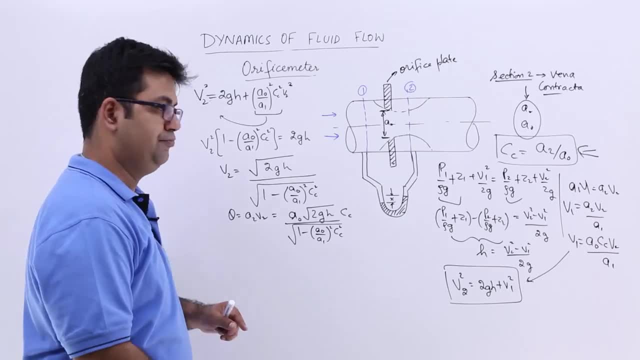 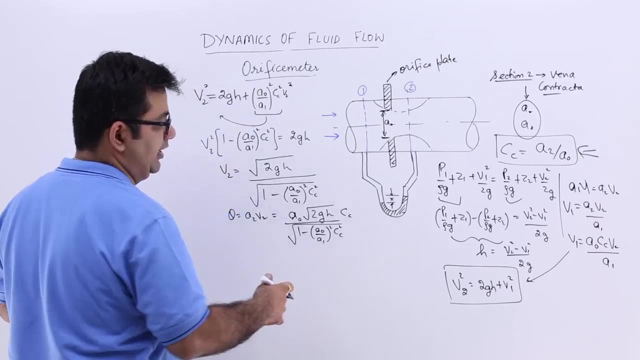 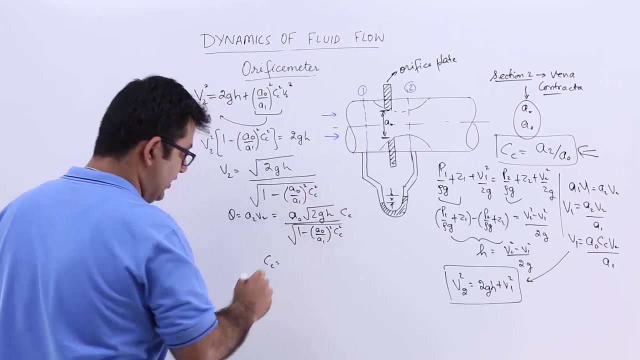 get a0 and there will be a cc over here. alright, now let's assume a term, let's assume a value, so that we can get rid of this and get a much simpler, you know, term in place of this. so let us say that this cc is equal to cd, that's the coefficient of discharge for the orifice. 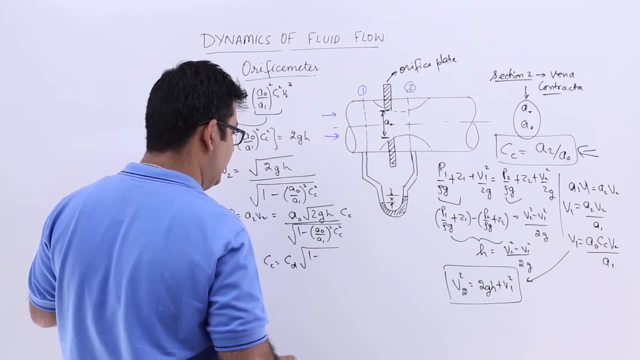 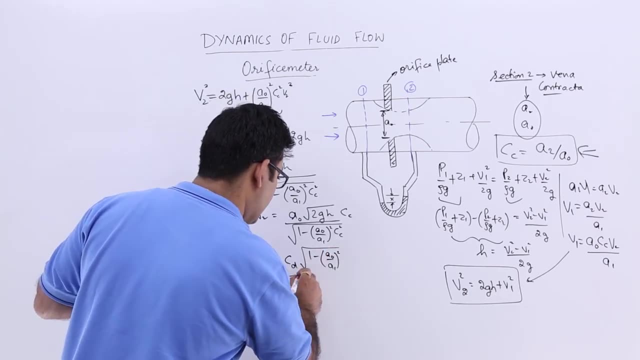 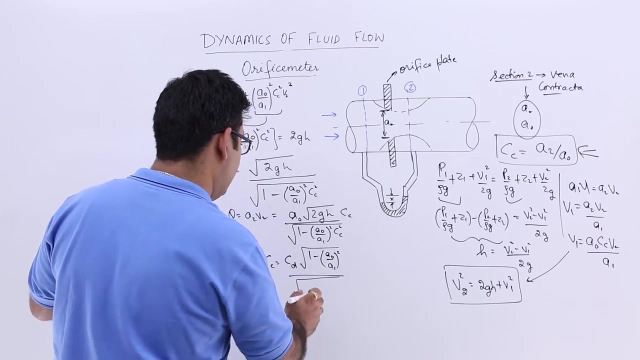 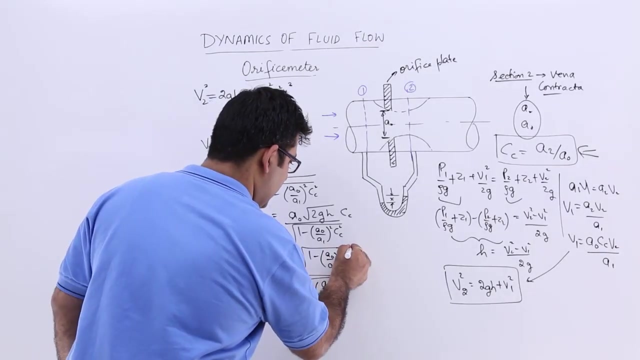 meter into under root. 1-. this will be a0 upon a1 whole square. upon. this would be into, you will get 1- a0 upon a1 whole square. so I will add another term, which is cc, square over here. okay, so now you have a substitution. 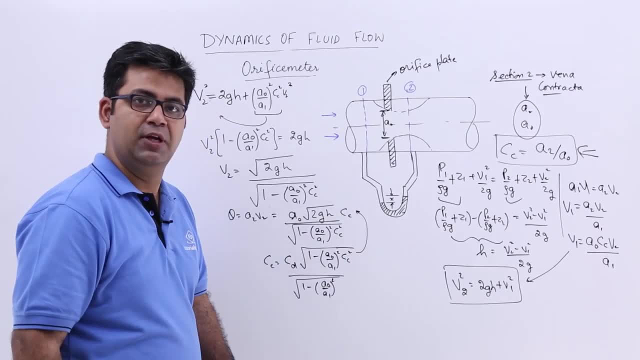 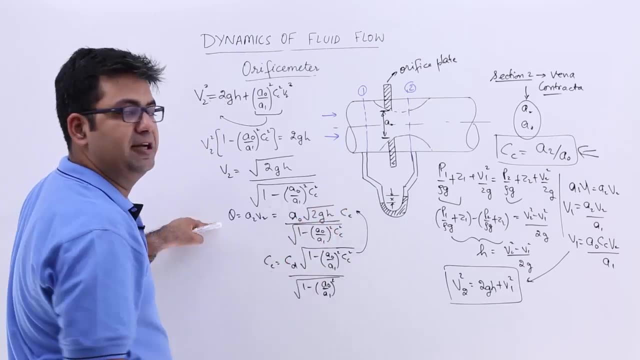 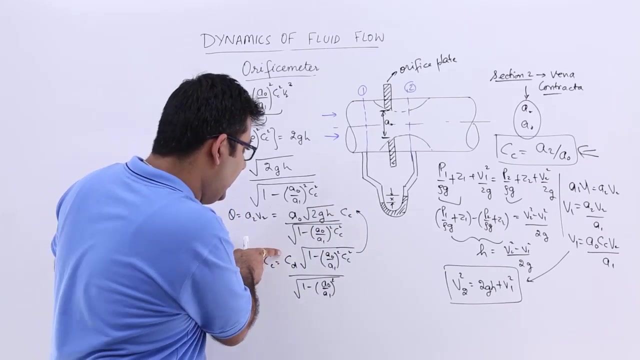 for this cc over here. so with the help of this substitution I will get a value for q which will not have cc in it. it will be taken care of in the numerator also and in the denominator also, because with this cd you have this term with cc square in the numerator, and this is 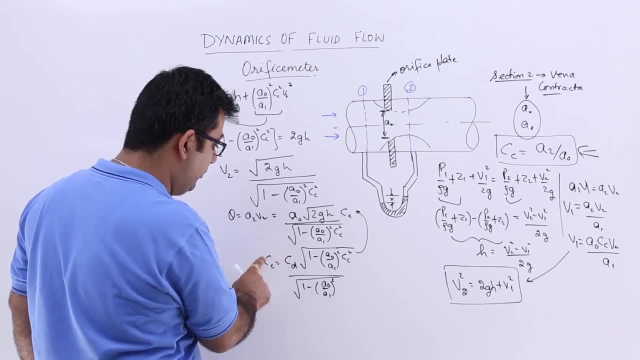 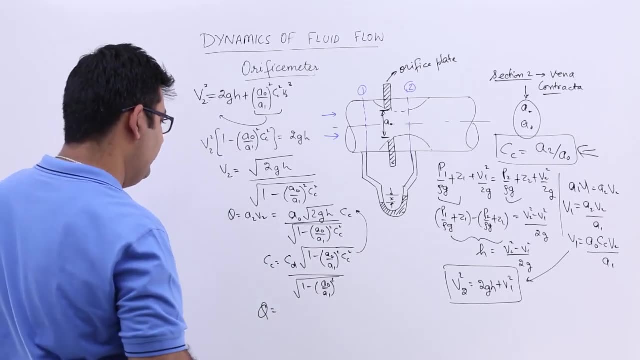 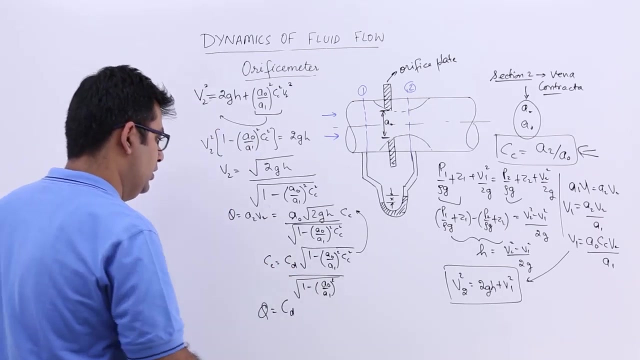 in the denominator. so these 2 terms will cancel when I put cc over here. alright, so when you do that now you get a value of q which is equal to, you'll have your a0. so I will put cd first of all. you'll have your a0. okay, and only this part will be left in the denominator and this: